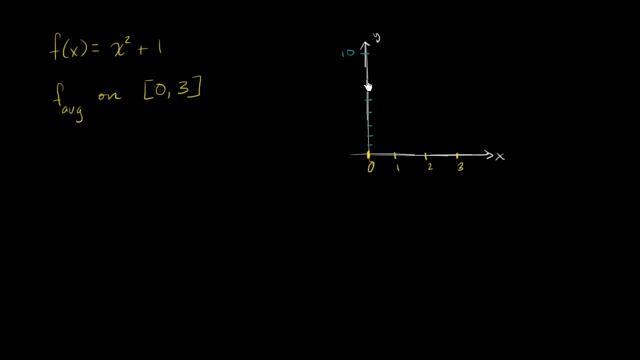 So let's see, This is gonna be in the middle, Pretty good. And then let's see in the middle, And then we have that. Oh, good enough, All right, So we're gonna be, we're gonna be there. 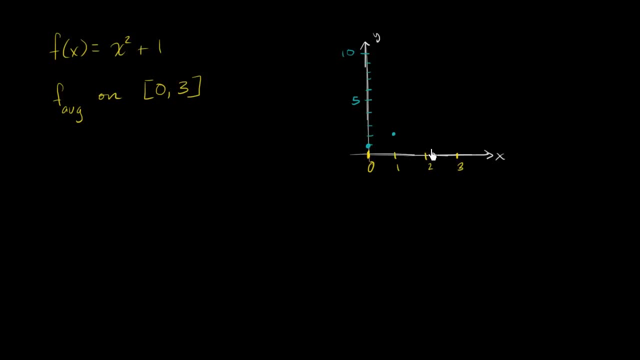 We're gonna be there. I have obviously different scales for x and y-axes. Two squared plus one is five. Three squared plus one is 10.. Three squared plus one is 10.. So it's gonna look something like this: 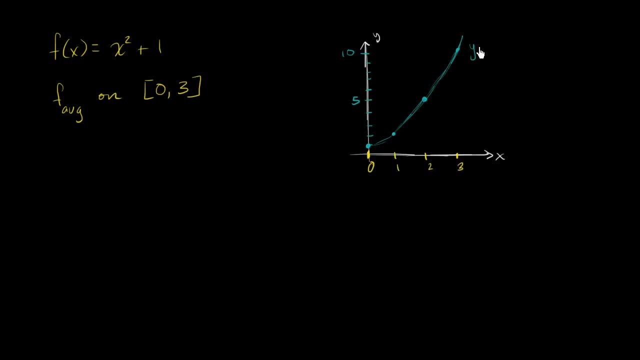 This is what our function is going to look like: Graph of y is equal to f of x And we care about the average value on the interval closed interval between zero and three, Between zero and three. So one way to think about it, you could apply the formula: 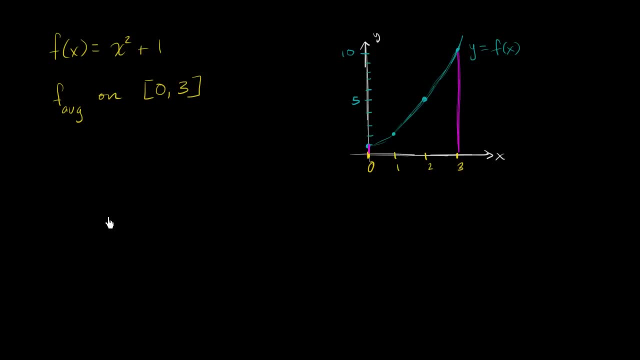 but it's very important to think about: what does that formula actually mean? And once again, you shouldn't memorize this formula because it actually kind of falls out out of what it actually means. So the average of our function is going to be. 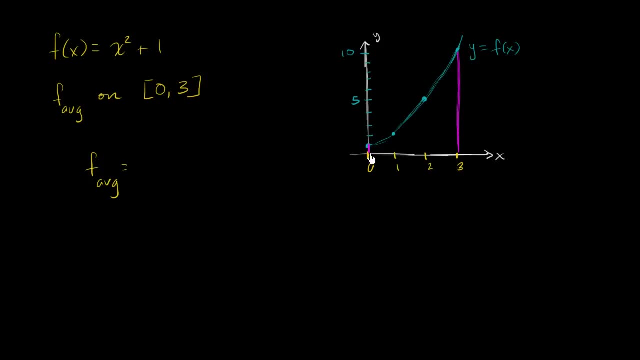 it's going to be equal to the definite integral over this interval, So essentially the area under this curve. So it's going to be the definite integral from zero to three of f, of x, which is x squared plus one dx. And then we're gonna take this area. 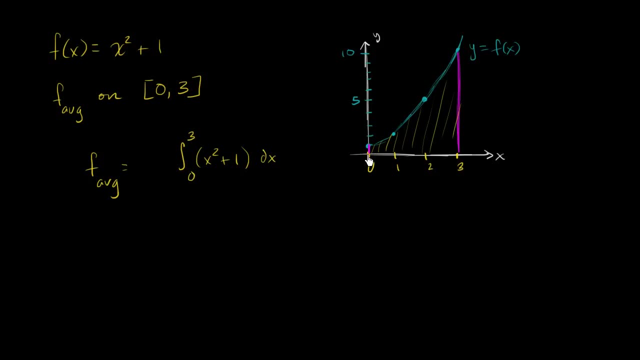 We're gonna take this area right over here And we're gonna divide it by the width of our interval to essentially come up with the average height or the average value of our function. So we're gonna divide it by b minus a or three minus a. 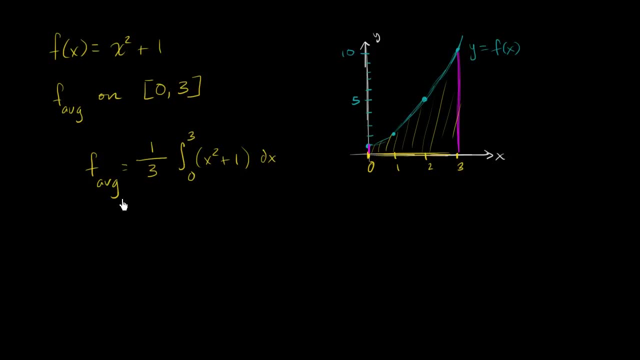 So that's zero, which is just going to be three, And so now we just have to evaluate this. So this is going to be equal to one third times. see: the antiderivative of x squared is x to the third over three. 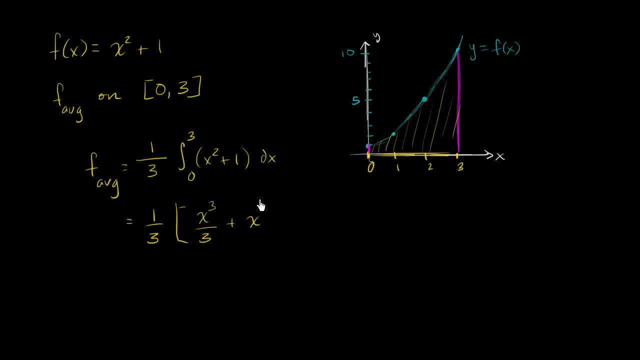 Antiderivative of one is x, And we're going to evaluate it from zero to three, And so this is going to be equal to one third times when we evaluate it at three- let me use another color here- When we evaluate it at three.